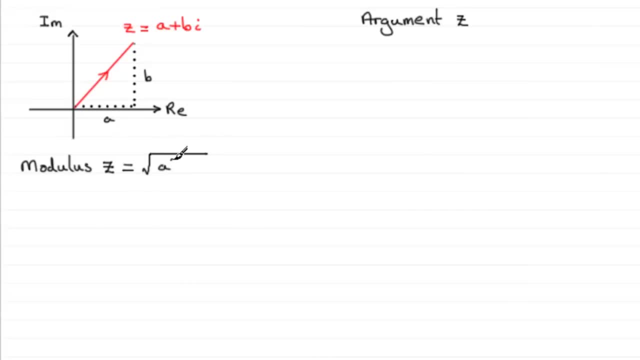 root, then of A squared plus B squared. Now there's various other notation that you can get for something like this. A very common one is to see this written: Okay, Z with two straight lines down the side, Often referred to as the mod of Z for short, And that too is going to obviously be equal. 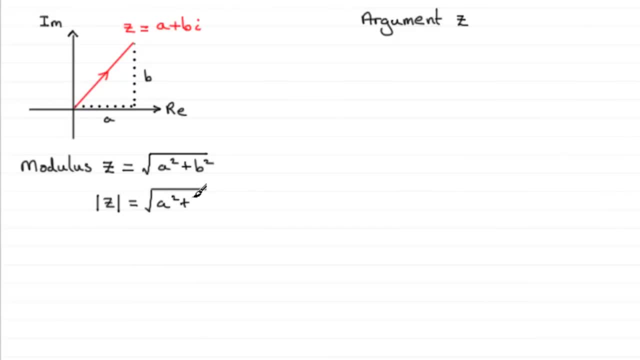 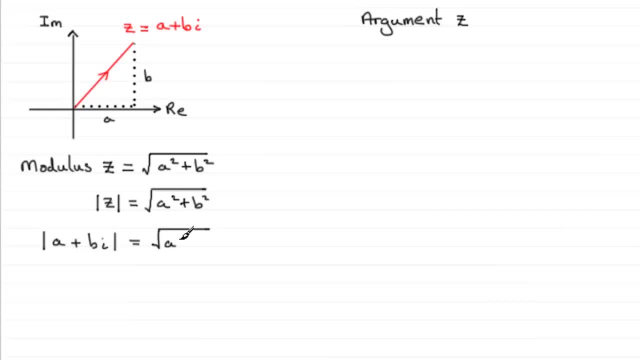 thing, the square root then, of a squared plus b squared. some authors just simply write mod Z. mod Z, then, will be the root of a squared plus b squared, and so on. another form that you can get is that the length of this can often be that denoted by, say, R, and if that's the case, then R is equal to the root of a. 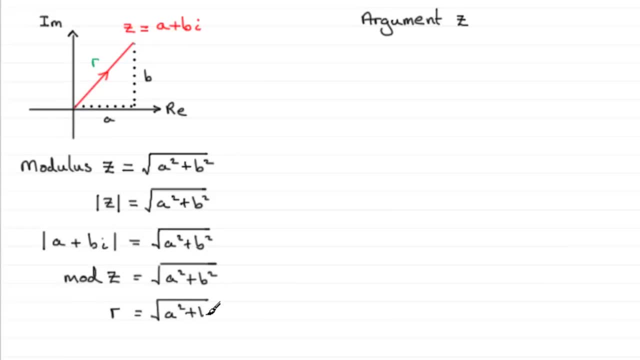 squared plus b squared. so quite a few different ways of writing down the same concept. ok, so what do we mean by the argument of Z? well, the argument of Z is an angle, it's an angle theta and on this diagram, it's the angle made between the positive real axis and 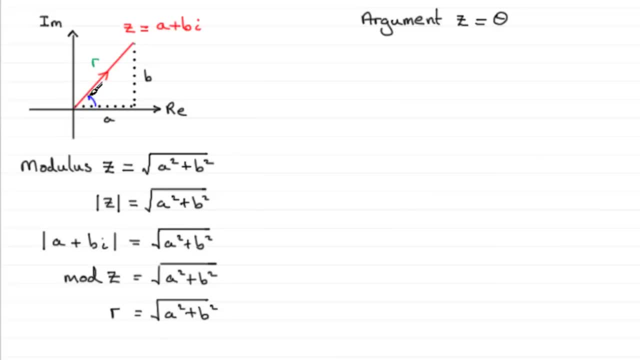 the complex number. so it would be this angle around here, but we've got to be careful with theta. it's normally measured in radians and it's an angle that goes between minus pi and it's less than or equal to pi. radians in degrees. that's obviously greater than minus 180 degrees but less than or equal to a. 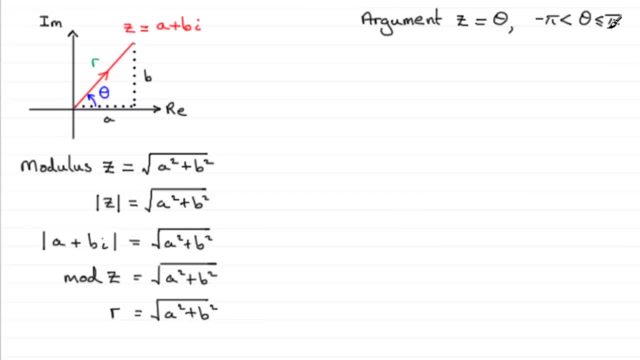 hundred and eighty degrees, but we tend to work in radians and for short, some people call this argz, so you can be seeing this quite often: argz equals this angle, theta. Now you've got to be careful because of this angle lying between these restrictions here. 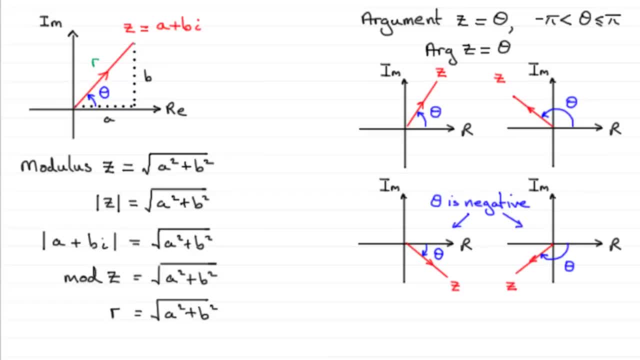 Because when you get complex numbers drawn, they can be in various quadrants: The first quadrant, second, third and fourth quadrant- And so you can see that I've marked on in each of these diagrams the arg of z, the angle theta. 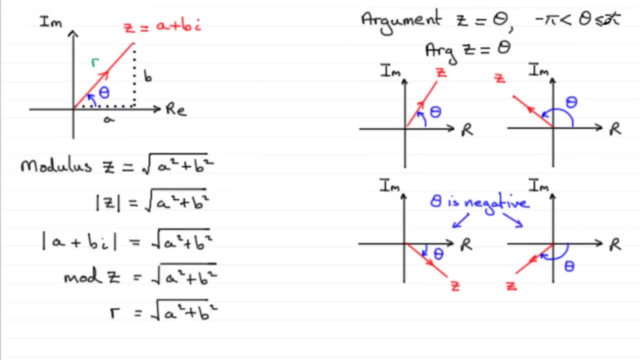 But because it's got to lie between minus pi and pi here, when it goes into this third quadrant or the fourth quadrant, we've got to turn in the negative sense. So theta will be negative. In these two it's always positive. 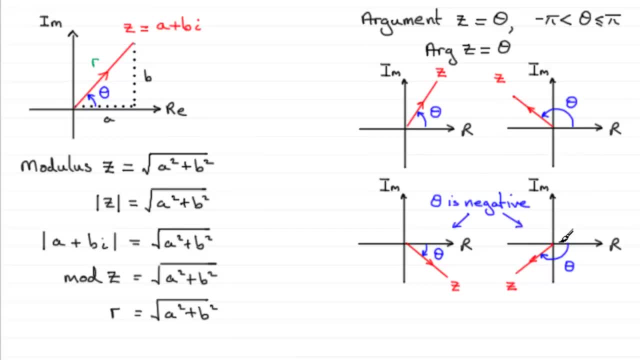 Now, how do we work out what this angle is? We can be very careful with this type of quadrants, Because what I would encourage you to do is always select the acute angle in any diagram. For this one, this is easy, because the acute angle here is theta itself. 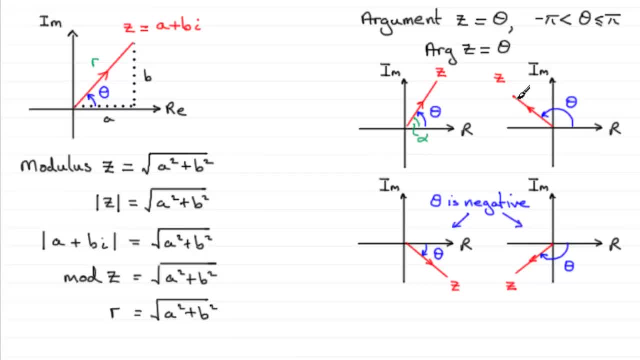 But I'm going to call it alpha. In this one, the acute angle here would be this one. here, This would be my alpha, And in this one, this would be alpha. And when you're finding the arg of a complex number z, always draw a sketch. 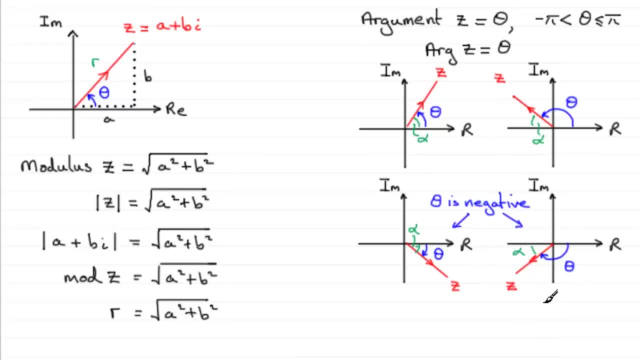 Otherwise you're going to get caught out, or likely to be caught out anyway, as you'll see later on in the examples that I do. And how do we work out this acute angle alpha? Well, again, we look back at the triangle that we can draw, the right angle triangle. 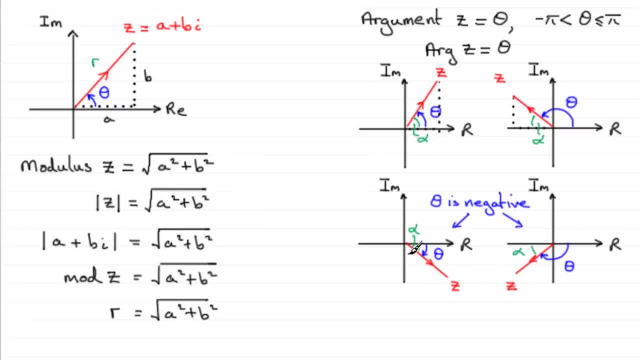 In each of these we'll have a right angle triangle looking something like this: OK, To get alpha. what we do is we look at what tan alpha equals. Tan alpha will always equal the opposite side over the adjacent side, Opposite over adjacent. 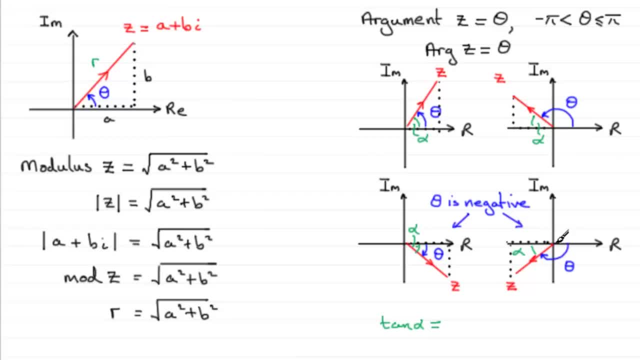 Opposite, over adjacent And so on. OK, But the lengths of these sides we take as the positive value of the a and the b that we've got for the complex number. In other words, we take the mod of b over the mod of a. I know I'm using the word mod, again very similar to what we. 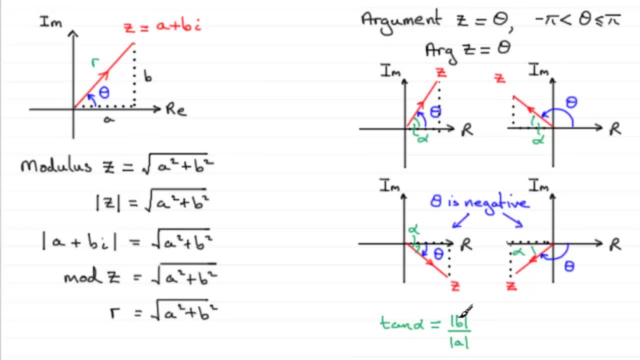 had here, but it's in the context of taking the length of these sides. So it follows that alpha will be equal to the inverse tan, then, or arctan of the magnitude of b over the magnitude of a, And once you've got alpha, for instance, you can work out what this theta. 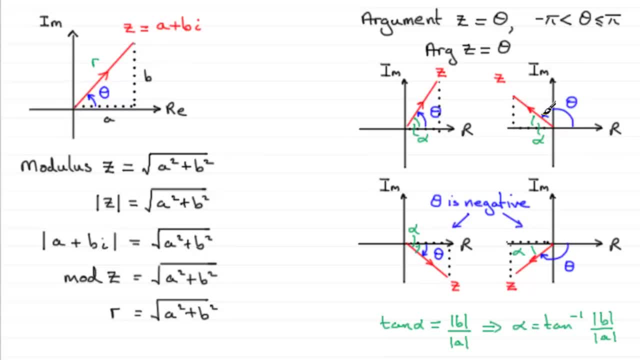 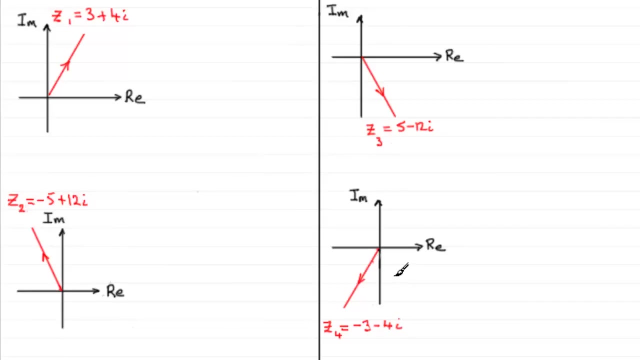 is by just doing pi radians minus alpha, And you should be able to get the various values of pi radians. Now, as I say, you've got to take care over these ones. But I've got an exercise here coming up. I've given you four questions that you can try and have a go. Just pause the. 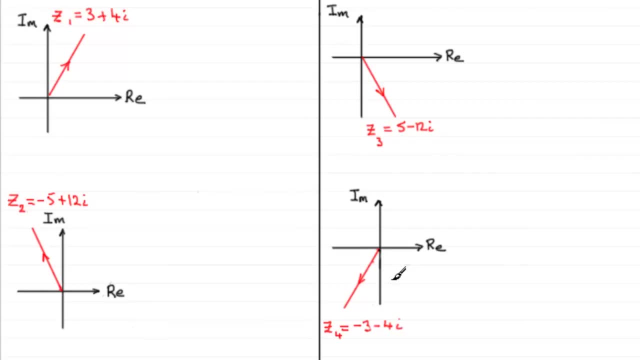 video and come back when ready and I'll work through the solutions. Okay, well, let's see how you got on, if you had a go. Well, the first one is fairly straightforward Because it's in the first quadrant. we haven't got to worry about positives and negatives so much. 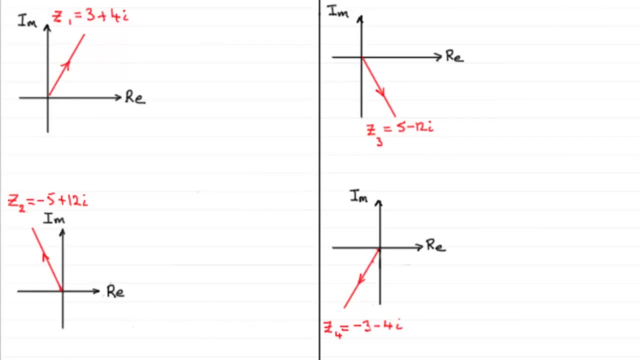 So, when it comes to working out the mod of z1,, all we need to do is think of our triangle through here. okay, This length up here will be four units. This will be three units. So when it comes to working out, then, the mod of z1, all we've got to do is use the 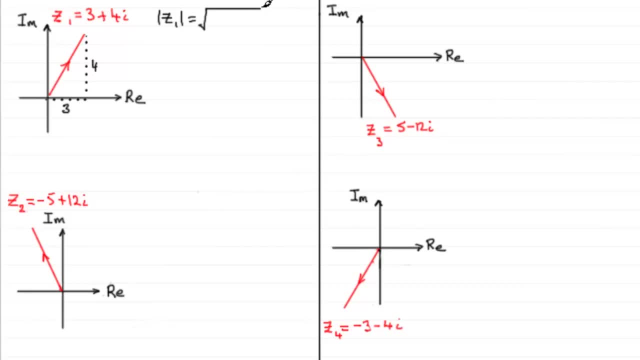 Pythagoras' Theorem, and it's going to be the square root then of 3 squared plus 4 squared. In fact, it's a well-known triangle. You should know that that's going to be the square root of 25, which is 5.. We often refer to it as the 3,, 4, 5 triangle. 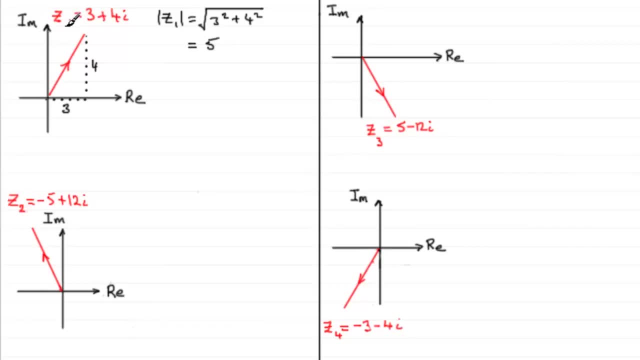 Now, when it comes to working out the arg of z1, that would be this angle here. Let's call it theta Now, because it's already an acute angle. I could actually go straight into this one and say that theta is equal to the inverse tan. 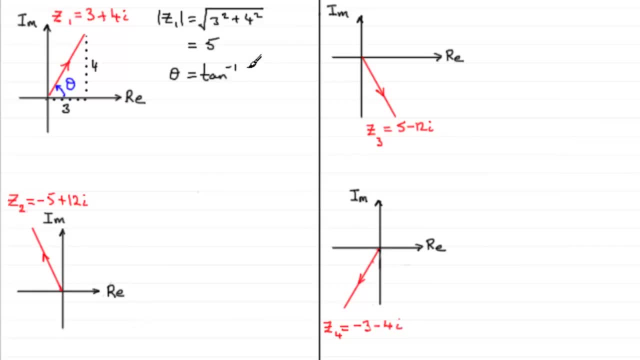 of 4 over 3, opposite over adjacent, And remember, we give this in radians unless we're told otherwise. And if you put your calculator in radians mode and do this, you'll end up with 0.927, and so on radians. 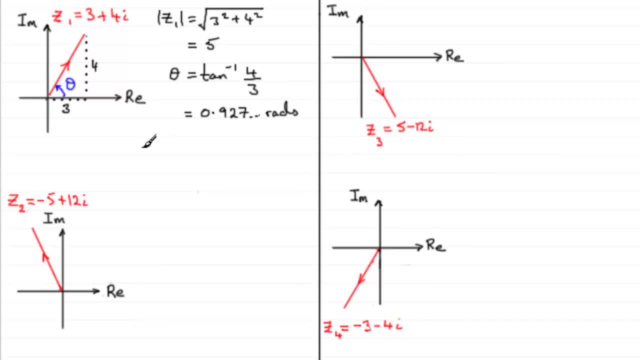 So when it comes to the arg of the complex number z1, we can say that, therefore, arg of z1 equals 0.9 radians, say, to one decimal place. Okay, so there's the first one. Now I want to turn our attention, in fact to say this one down here, rather than going to this one. 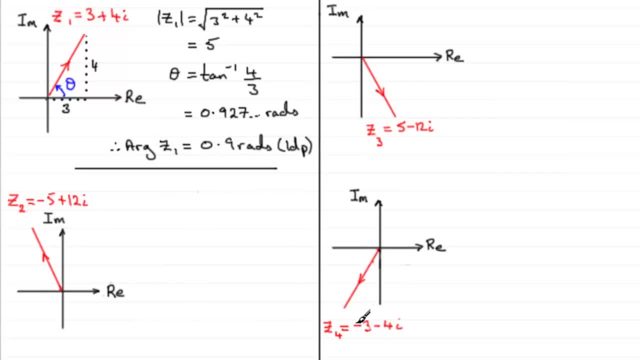 because you can see I've used the same numbers here essentially as I've used up here, And I'll show you why. it's important to work out acute angles in a moment, But when it comes to working out the mod of z4,. 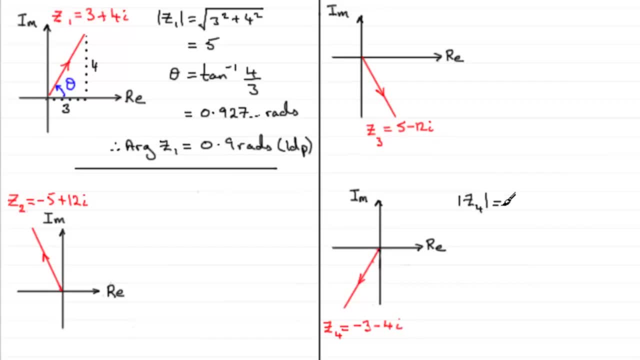 the mod of z4 is going to be essentially exactly the same as what we had up here. We'll draw our triangle in, say Okay, let's just put that in, And we've got our lengths as being 4 units downwards and 3 units to the left. 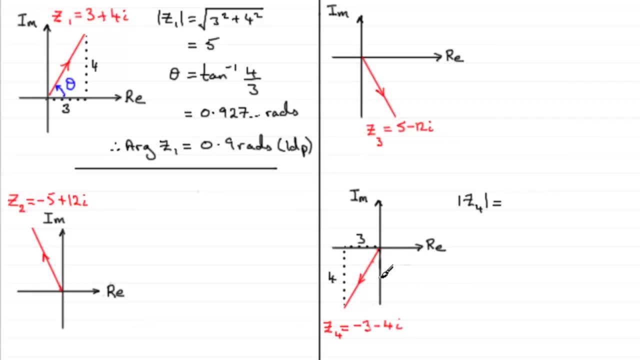 So when we work out the mod of z4, we've got our triangle again, just like we had up here. It's going to be the square root of 3 squared plus 4 squared. Now you could write minus 3, as long as you write minus 3 in a bracket, all squared. 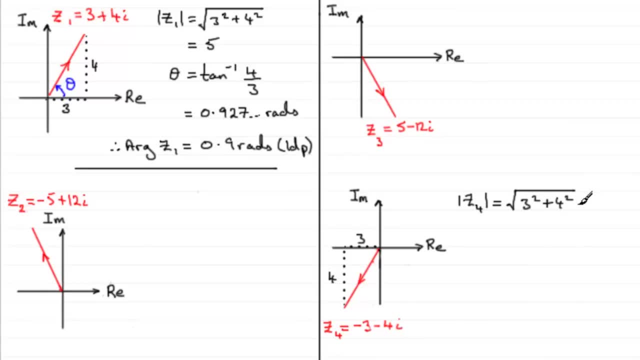 Plus negative 4 all squared. Same thing, though. Okay, I tend to take off my minus signs when I'm dealing with negative values. I'm only concerned with the lengths of the sides of the triangle. Anyway, we know that this one comes to 5, the root of 25 being 5.. 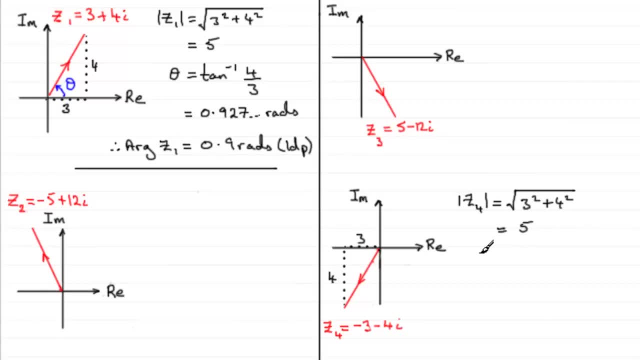 But when it comes to working out arg of z4, then we need to be thinking about working out this angle round here which is going to be a negative term- Let's call it theta then- But we need to work out what this angle in here is. 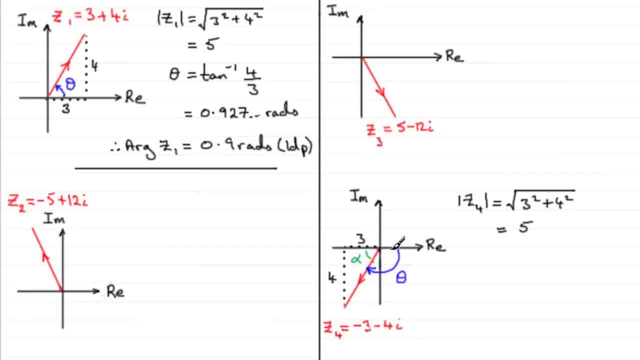 this acute angle is which I'll call alpha. So when we work out alpha, we know that alpha is the inverse tan or arctan then, of the 4 over 3. And we know that that comes to because we worked it out up here. 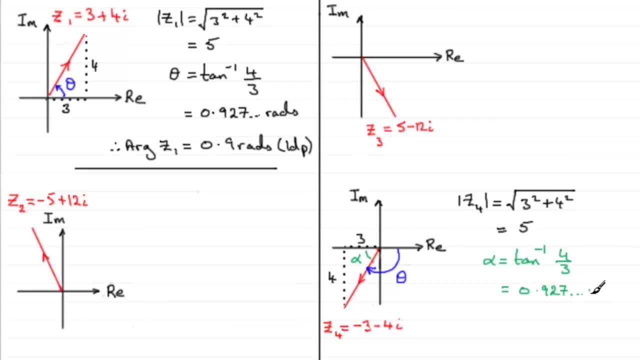 0.927, and so on. radians. So, when it comes to working out what the arg of z is, we therefore have arg of z4.. Well, that's going to be equal to a minus angle, and it's going to be pi minus the 0.927 and so on. radians. 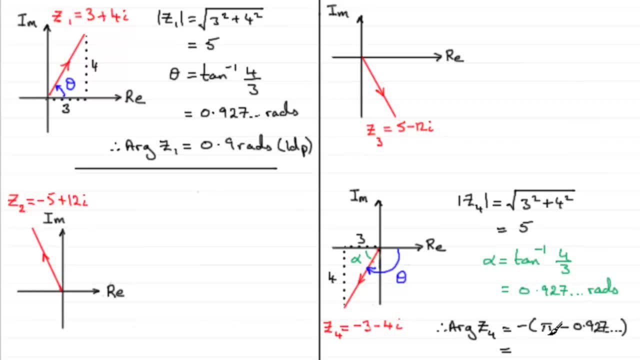 Now, because I'm running out of room, I'm going to round this up. What you get is minus 2.2 radians to one decimal place. So you've got to take care over these, because it's so easy just to say: 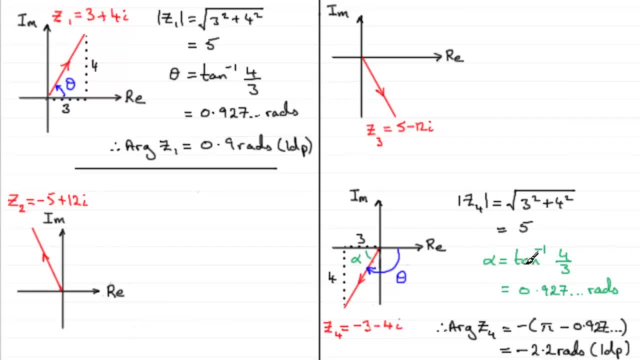 that the arg is equal to the inverse tan of the imaginary number over the real number, And if you did that, you'd have minus 4 over minus 3, which would give you exactly the same result as this, But it's not really minus 4 over minus 3.. 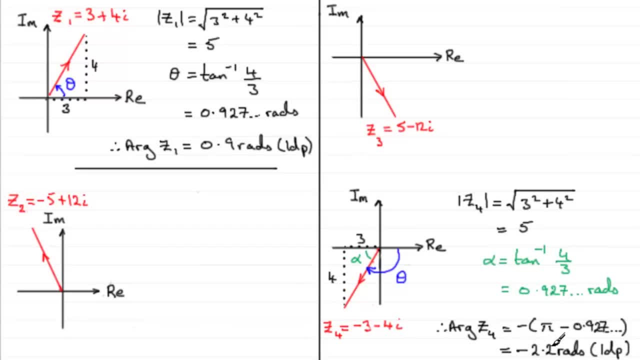 As you can see, it turns out to be the minus 2.2 radians. Okay, well, let's see how you got on with, say, this one over here. Same way, we would draw ourselves a triangle round here and our lengths would go in as 12 units up, 5 units to the left. 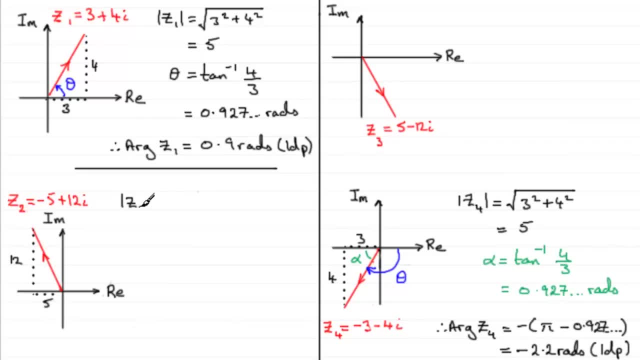 When it comes to the mod of z2, this is a familiar triangle. if we're using Pythagoras' theorem, This is what we call a 5-12-13 triangle. But if I was working it out and didn't know that, 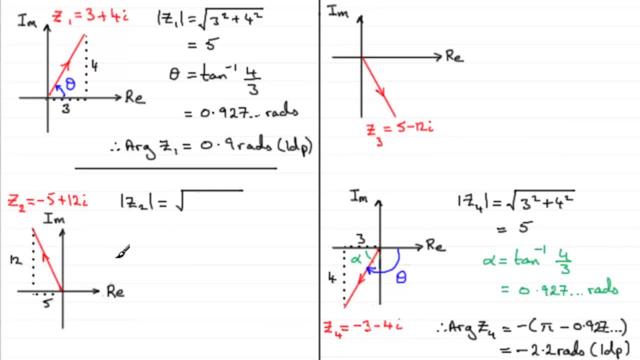 then I could either write: 5 squared plus 12 squared- but I'm going to strip off that minus because I'm only concerned with lengths. so it's 5 squared plus 12 squared, The square root of 169, which is 13.. 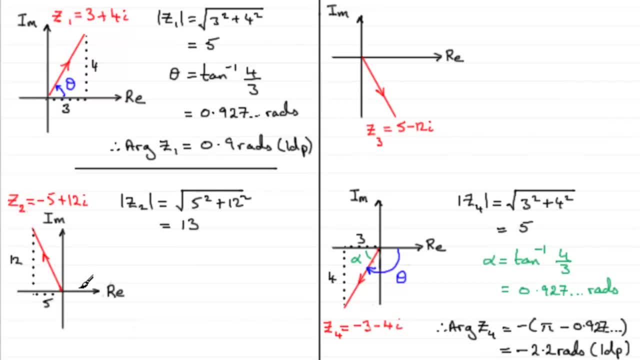 And when it comes to working out what arg of z2 is, we're looking at this angle round here, which is going to be a positive angle, But to get it, I would look at this acute angle in here, alpha, and if you work that out, 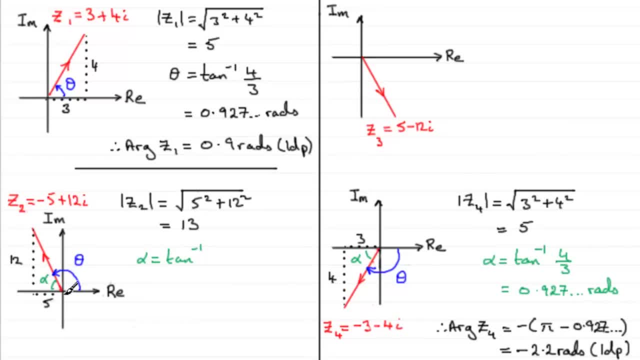 alpha equals the inverse tan of 12 over 5.. Remember to be in radians mode and if you work that out in your calculator, you'll find you get 1.176 and so on, radians. So when it comes to working out what theta is, 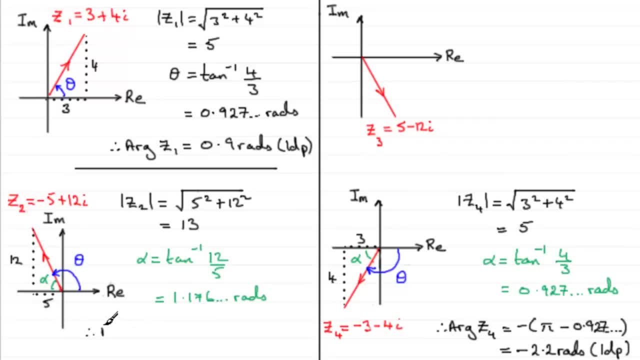 the arg of z2, then we've just got to say: theta equals pi radians minus alpha, pi minus then 1.176 and so on, And if you work that out and round it up you'll find that you get 2.0 radians. 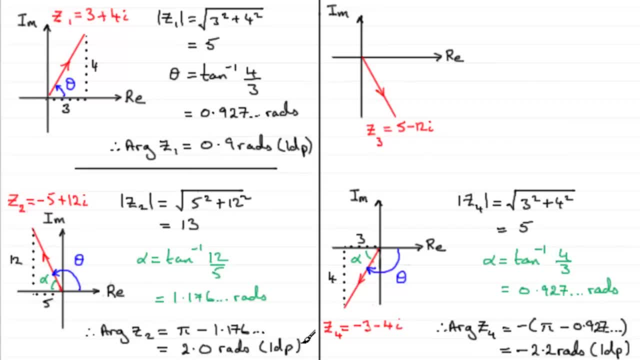 okay, to one decimal place. And similarly I've got another complex number here: same values, basically the 5 and the minus 12.. If we draw our triangle in here again, like so, we can see that this length is 5 units.